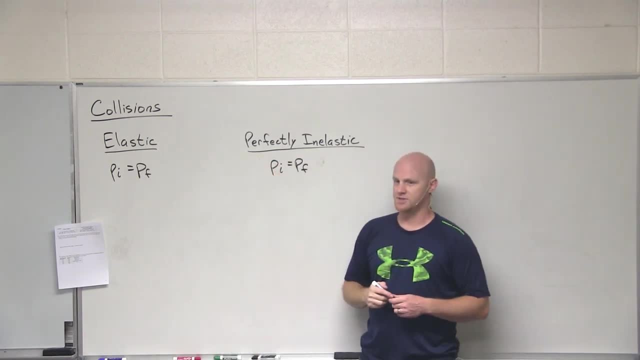 Momentum is always conserved before and after collision, So you could look at it in that context. So, but in this case, you just definitely, definitely need to know that momentum is always conserved. It doesn't matter the kind of collision. 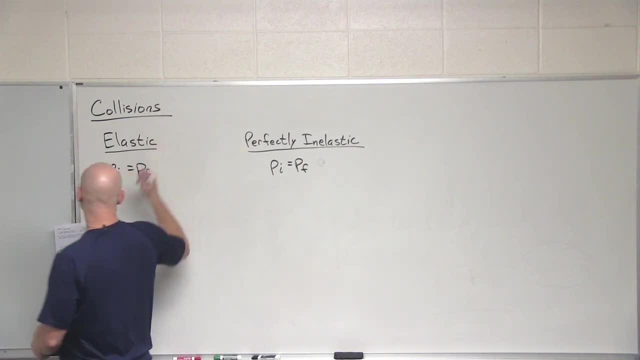 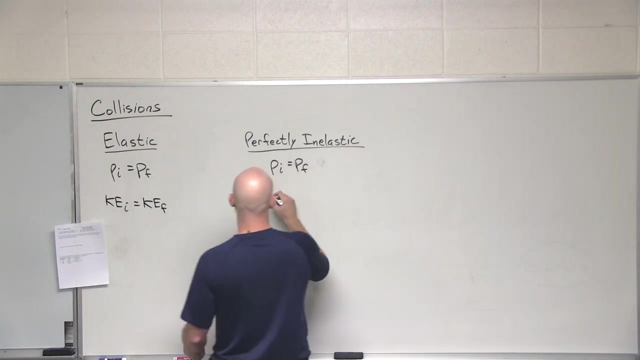 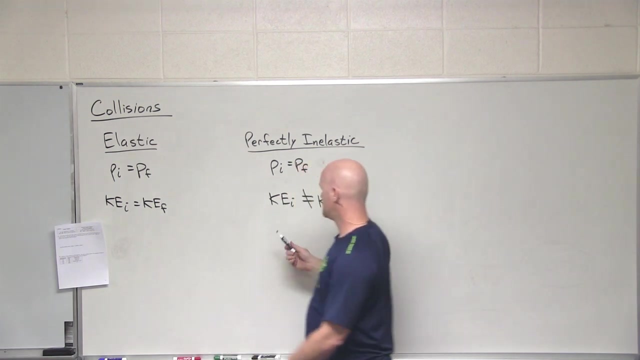 What's not necessarily conserved is kinetic energy. For an elastic collision, kinetic energy is also conserved, So, but for inelastic collisions, whether it be just plain old inelastic or perfectly inelastic, kinetic energy is not conserved. So 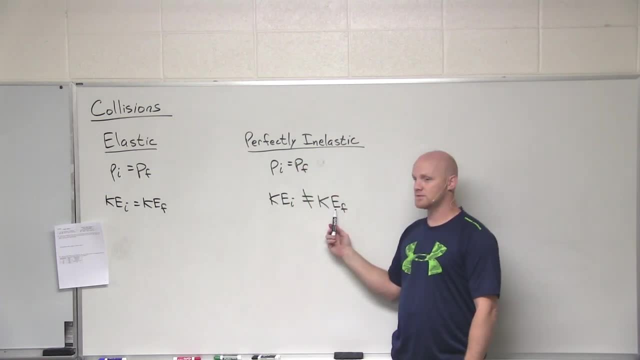 your initial and final are never the same. Your final is always not necessarily zero, but less smaller. You always end up with less kinetic energy. So in inelastic collisions you always lose kinetic energy. So in a perfectly inelastic collision, 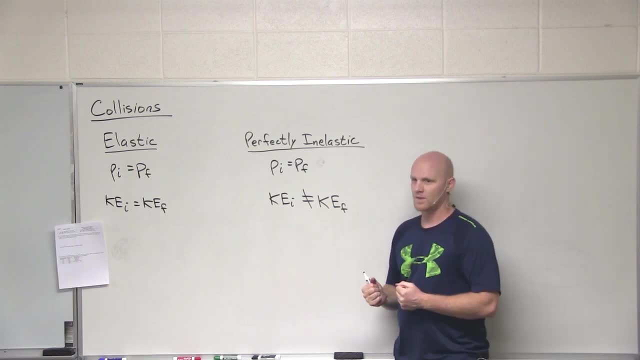 the amount of kinetic energy you've lost is at a maximum In a plain old inelastic. you haven't necessarily lost the maximum, but you've lost a fair amount. Now, the hallmark of a perfectly inelastic collision is that the two objects that have collided, or if there's more, 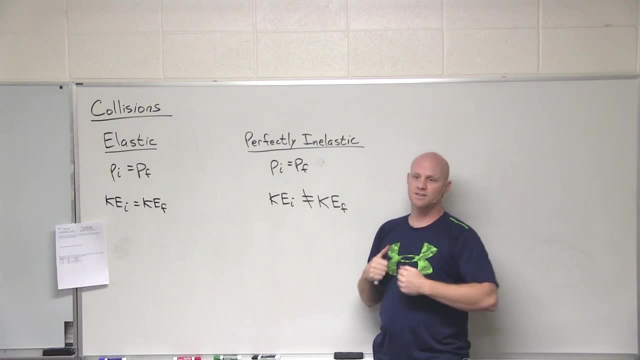 than two. but in the case of two objects colliding, they are stuck together. If they stick together you have a perfectly inelastic collision. If two objects collide and have no propensity to stick to each other, no propensity for any kind of permanent deformation or anything like that. 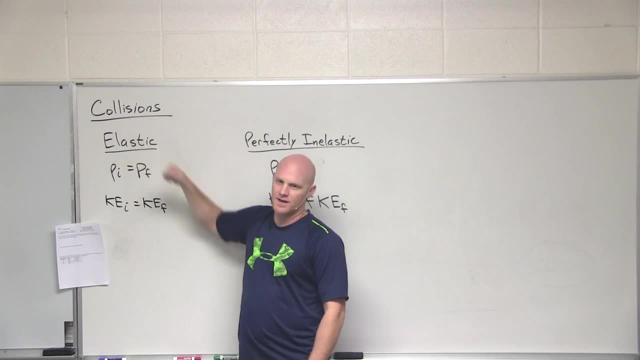 that's probably where you're gonna get as close to an elastic collision as you can come, And the classic example is billiard balls colliding on a pool table. So do you? Yeah, billiards, Sweet. So these billiard balls on a pool table, are they? Do they have any propensity to stick to each other? 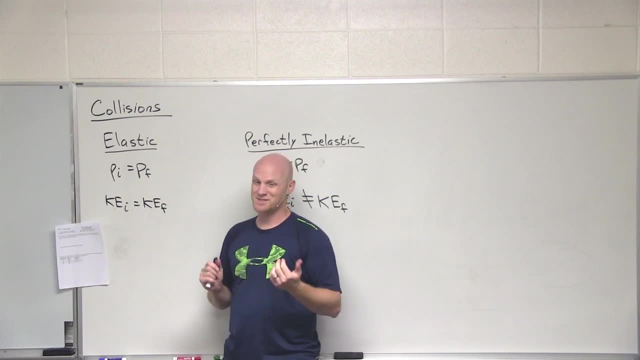 Not really Do. they deform upon collision much, Not much at all, Hardly noticeable amount, And so that would be as close. you know, it's kind of a textbook example of an elastic collision. So the truth is, though, there's no such thing as something that's completely, perfectly, absolutely elastic. 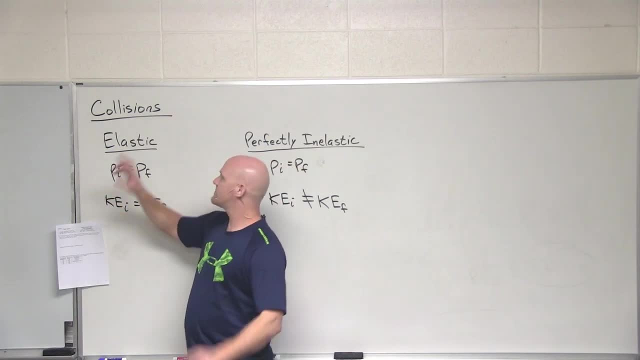 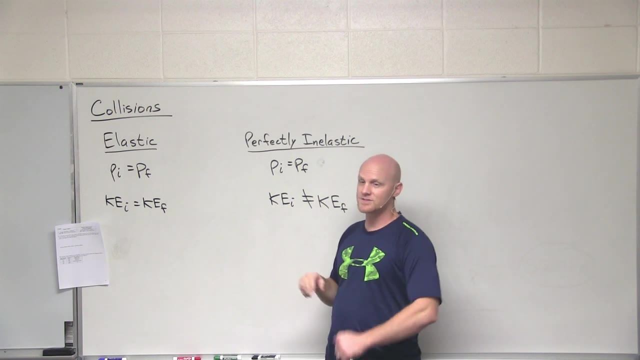 Just our best approximations. So, and in this case, for our theoretical elastic collisions, yes, kinetic energy will be conserved. For every other, For every other kind of collision, whether it be plain old, inelastic or perfectly inelastic, you're always gonna lose some kinetic energy.